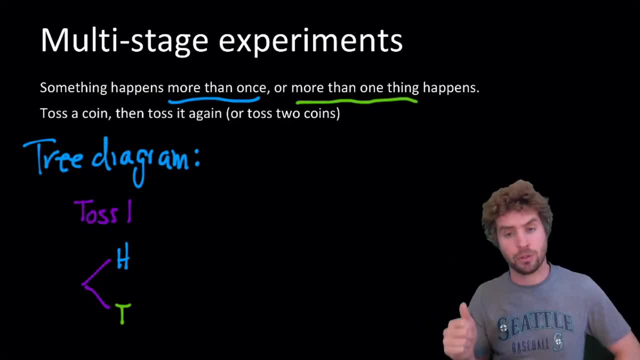 Okay, So we have our toss number one: Right, We flip the first coin To flip the coin the first time- Right, And the different outcomes that can happen are heads and tails- Right, And then for each of those outcomes, when we toss the coin again, there are another two potential outcomes. Right, There's heads and tails the second time. So in this, what we have here is heads the first time and then, potentially, heads or tails the second time- Right. Likewise, if we got tails the first time, we're going to toss the coin again- Right, And then for each of those outcomes, when we toss the coin again, there are another two potential outcomes. Right, There's heads and tails the second time. So in this, what we have here is heads the first time and then, potentially, heads or tails the second time- Right. Likewise, if we got tails the first time, we're going to toss the coin again- Right, And then, for each of those outcomes, when we toss the coin again, there are another two potential outcomes Right. 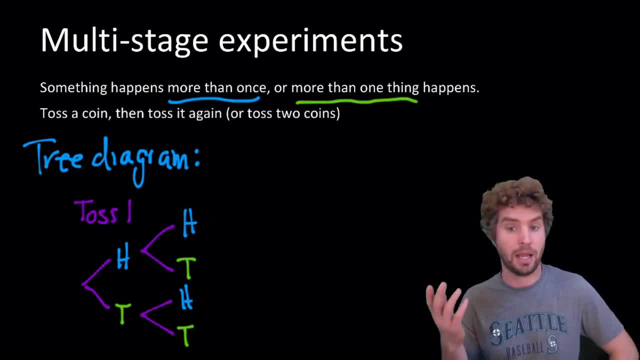 Likewise, if we got heads the first time, we can then get heads or tails after that as well, Right? So that's toss number two, coin flip number two or whatever, And what we can then do is diagram. We can make a list of all the sort of sequences, of what can potentially happen, Right, We can list all the outcomes of this two-step experiment, Right? So the first is that we have heads first and then heads again on the second roll. So heads and then heads, Right? Or we could go heads and then tails, Right. 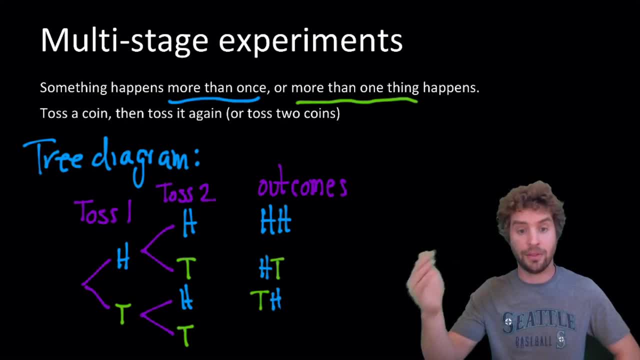 So heads, tails, Or we could start with tails and then heads, Or we could get tails both times. Right? These are the four possible outcomes of our experiment. Now, these two in the middle, the heads, and then tails, and tails and heads. if we're not concerned about the order of when they happen, then these are effectively the same outcome. Right, It's A heads and A tails. Right? 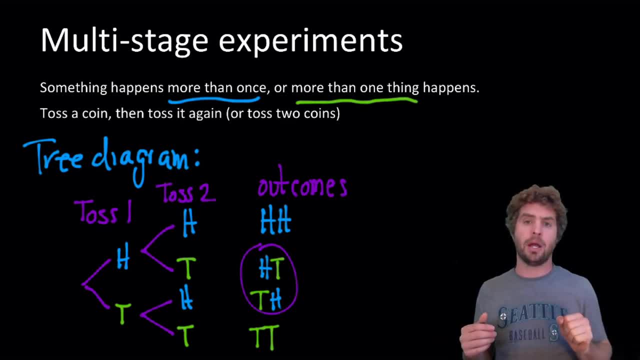 Followed by tails: Heads first and then tails. There's only one of those. But if they just say, well, what are the chances of getting one of each? There's two opportunities for that to happen. Okay, So two out of the total four. So that sequence you know of A heads and A tails, that combination, I should say, is a 50% chance, you know, of getting one of each. Right, It's 50-50 to get one of each heads and tails. 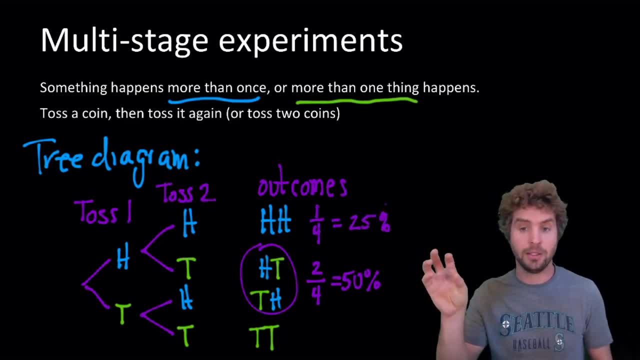 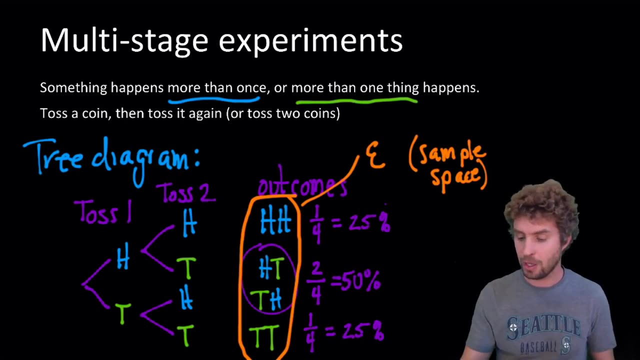 Whereas there's only one scenario with both heads out of the four. So that's 25% chance And same with two tails. Chances are 25% for that. This, of course, this list of outcomes, is our sample space, Right With the sigma Okay, And there are four things in the sample space. So the number as we have here, the number in the sample space, is four, Right, Okay. 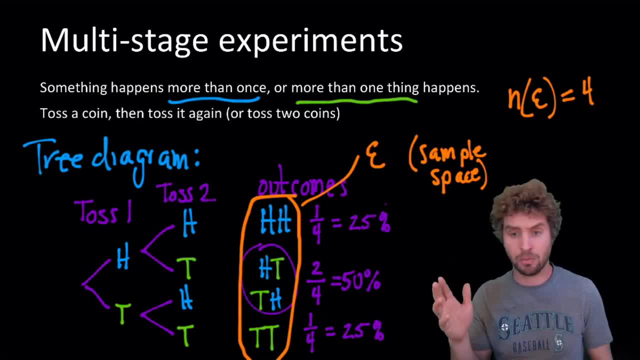 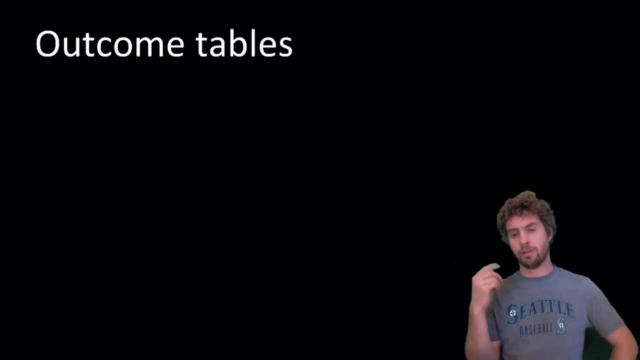 That's pretty much the idea. That's how it goes. It can get a little more complex. We can have things with more than two- you know outcomes for each trial or whatever- And we can have things. we can do things more than twice as well. So we'll look at a little bit of each of those, Okay, And for the next scenario, we're going to look at outcome tables and why we might want to use outcome tables. For example, if we're rolling a dice, okay, or a die or whatever. however, we say that the different outcomes in one roll are the same. 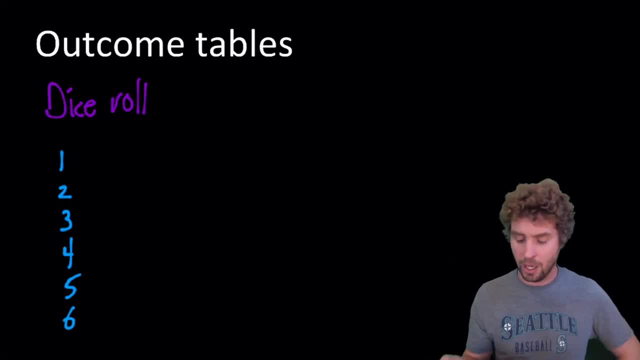 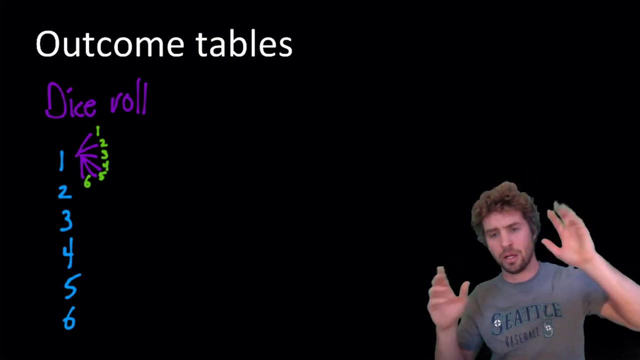 Our one, two, three, four, five and six. Right Now we can make a tree diagram for that. Right After the one, if you rolled another die, if you rolled it again or rolled a second one, then the second you know set of outcomes will be one, two, three, four, five and six as well. Right Now. that's going to get pretty cumbersome And making a table with that you either have to have really long lines or whatever, And it's going to get a little bit complex. 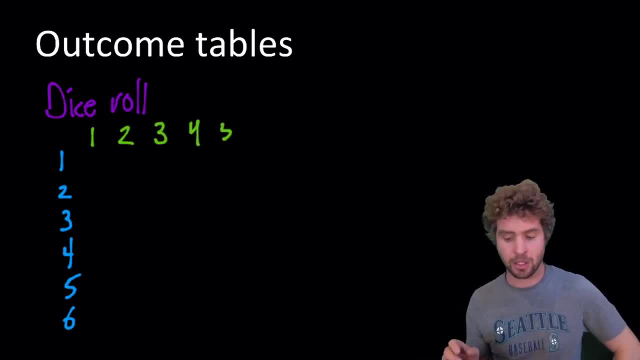 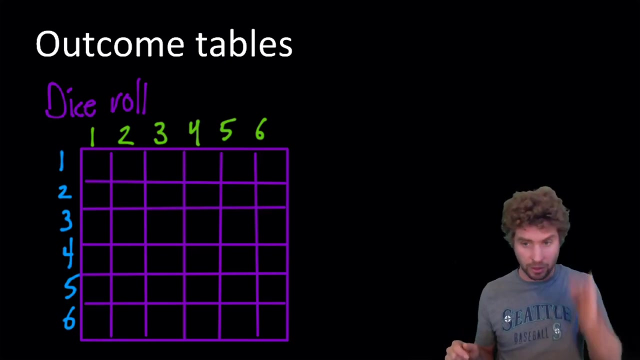 Another way to do that. this is with, as advertised, the outcome tables, And what we do is we put the second set of outcomes along the top right, at an alternate sort of sides of what we're going to have here, which is a big box, a table. Okay, So we make our table And you notice there's a column for each of the second, you know, set of outcomes And there's a row for each of the first set of outcomes. So we can take the ones, the one from the first roll and the one from the second- and put those together And then we can make a table with that. 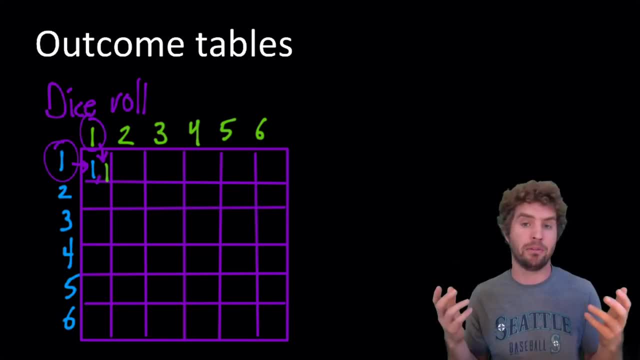 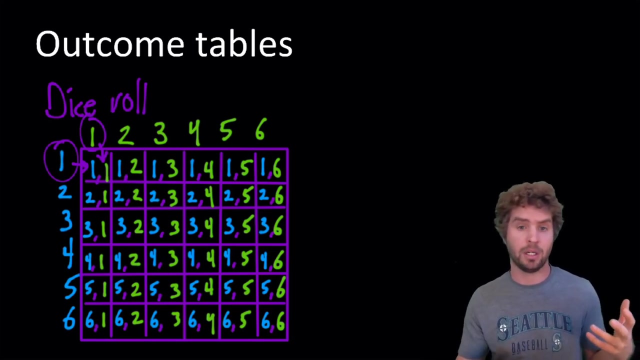 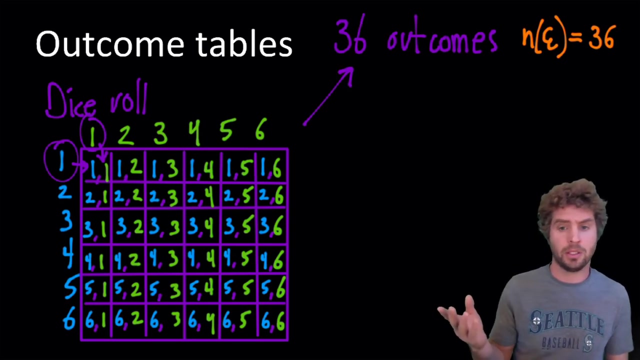 And then we can take the ones, the one from the first roll and the one from the second, and put those together, And then we can make a table with that. And then we can take the ones, the one from the first roll and the one from the second- and put those together, And then we can make a table with that. 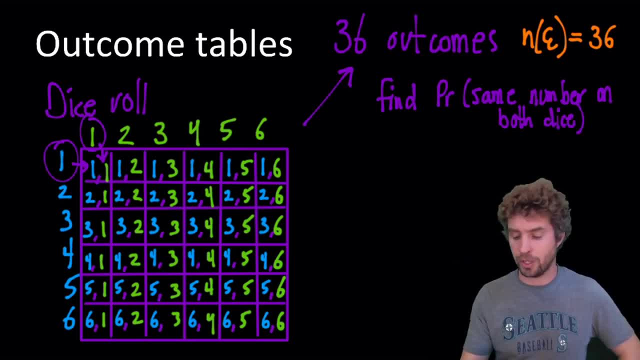 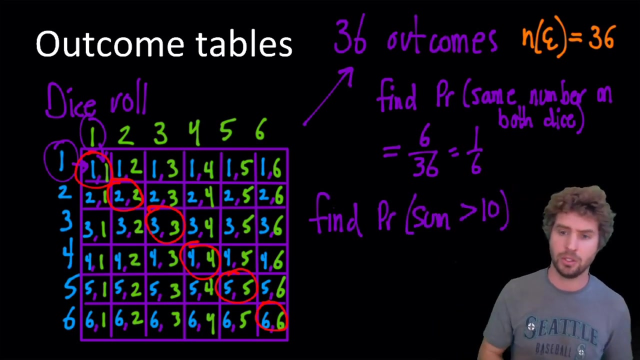 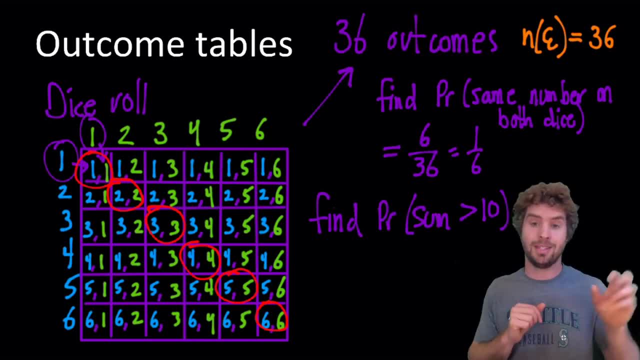 of the two numbers on the dice is greater than 10, right, more than 10. not equal to 10, but greater. so if we take the two numbers, add them together, what are the chances that gives us more than 10? well, we'll want to start down on the 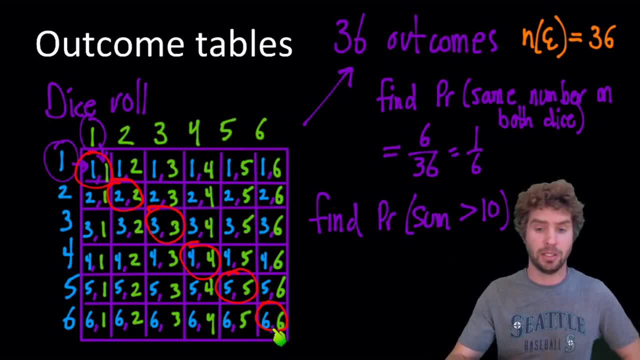 upper end. you know down here where the numbers are the highest right. 6 plus 6 is more than more than 10. 6 plus 5 is also more than 10. so there are these three different options. but then every other box, you know, either adds to 10 or 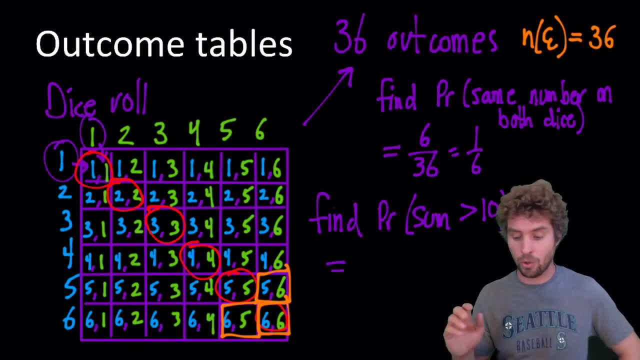 to something less than 10. so there's the three total options out of our 36, right, so that simplifies to 1, 12th. okay, and again you can calculate the percentage on calculator or whatever, if you want. all right, so outcome tables rather than.